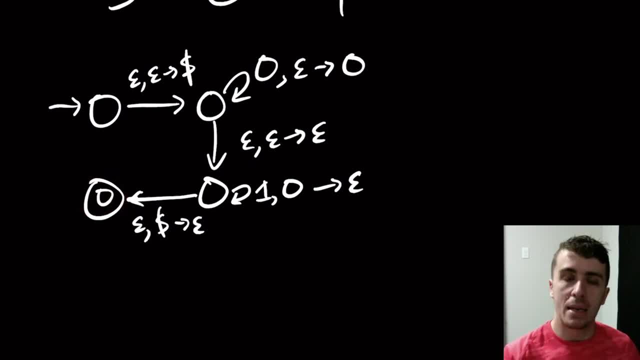 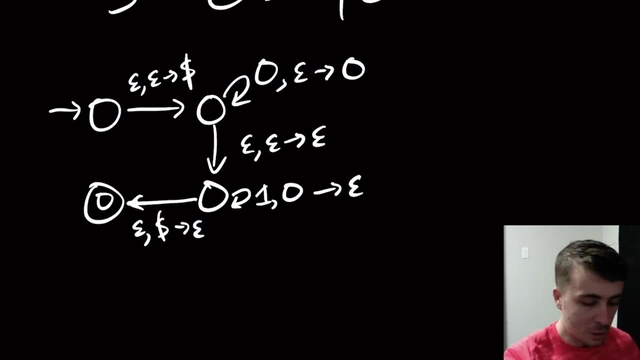 ends empty, which is one of the steps we had to do. But I'm not going to try to make this, I'm not trying to think very carefully about this. I want to be able to apply this without thinking at all. Okay, And the other thing we've got to make sure of is that we have no transitions that do. 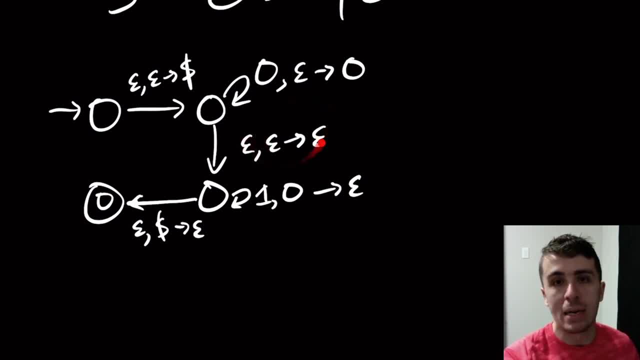 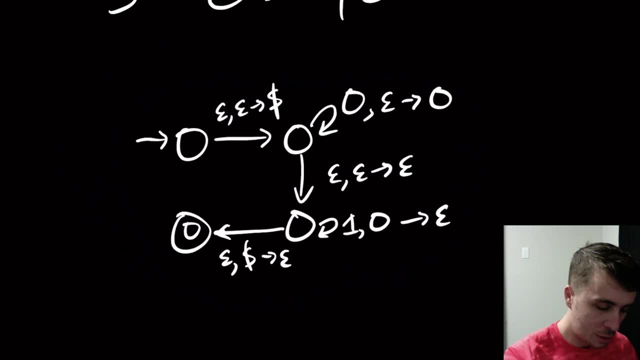 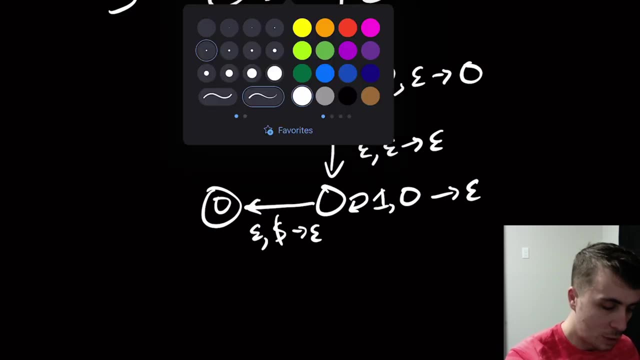 neither push nor pop or both, And we certainly have one right here. So let's make the modifications that we need. So I'm going to move this, So I'm going to move this over here, So we have some room, And so let's do the first thing, which is that 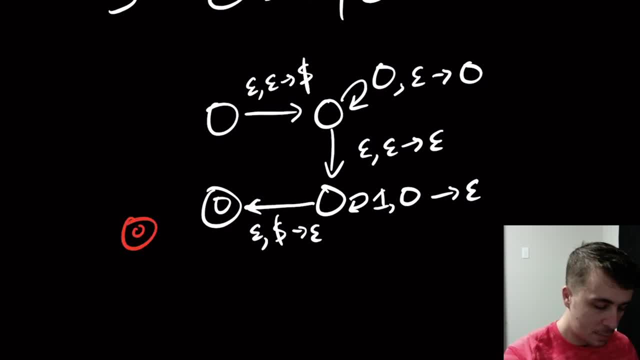 we have a single final state. Well, we already have a single final state, but what I'm going to do is just apply the construction that we did without thinking about, like, the structure of this PDA. So here we have again a triple epsilon transition. 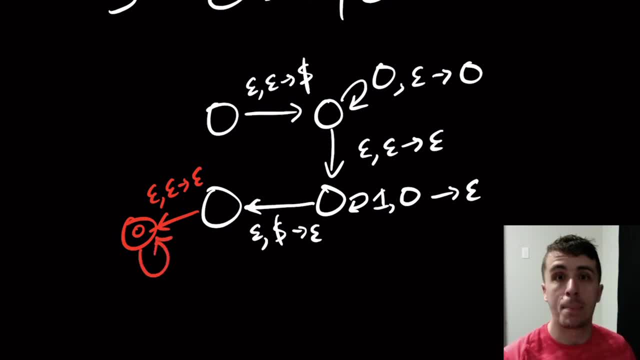 This state right here will self-loop and pop off anything that is not this new special symbol we're going to be putting in in a second. So the symbols that are used in the stack are the dollar sign and the zero. So here I'm going to have epsilon. dollar sign goes to epsilon so that it can pop. 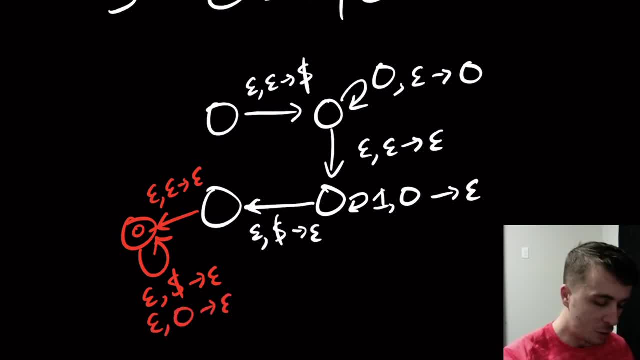 off the dollar signs if needed, and pop off zeros if needed. And then, once we do that, then we need to- or at least this is what we did in the construction- go to a new final state which is going to have epsilon and a new symbol. I'm going to call it pound sign because we've already used dollar sign. 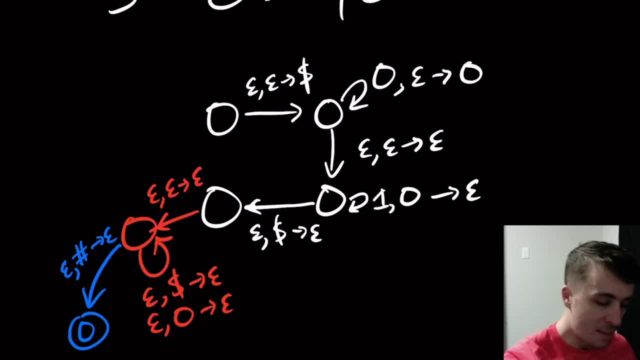 earlier and have it be popped off there. So then at the very beginning, the new start state is going to go to the old start state and push on that new symbol And then, once we do that, we're going to have a new special symbol And we can easily see that the behavior is unchanged, because the transitions 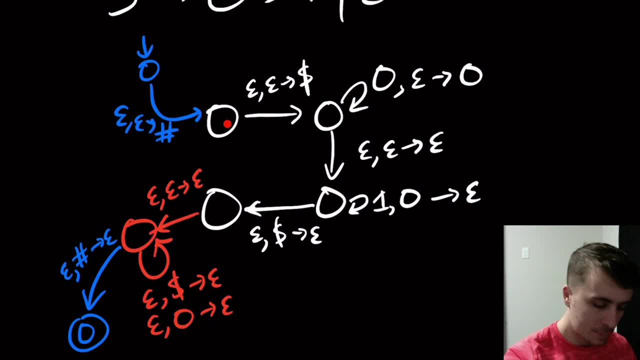 we add: don't read anything, so that's not affected. And once we push on a dollar sign here, then we're going to do the zero one business and then we'll come back here. So from here, if we have a string of zeros and ones- an equal number, we'll end up right here, having read the whole thing, with an. 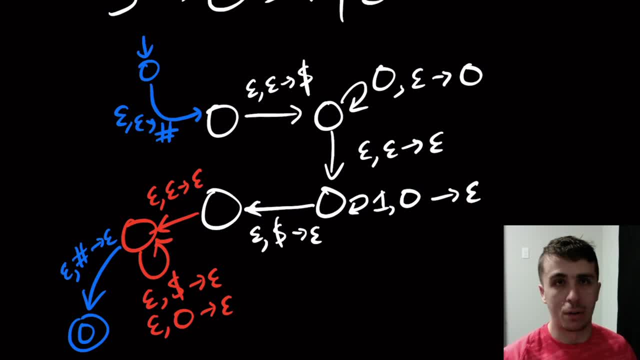 equal number, Hopefully, and although we've talked about reasons why it wouldn't actually matter if it wasn't exactly zeros and ones match, but- and that's unchanged here too, So this will allow us to pop off anything off the stack if we want to. that is not the new symbol, And then this will ensure that. 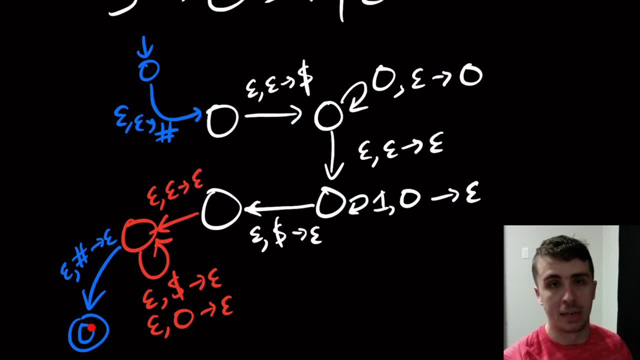 we will have the stack empty when we come down here. The only the other change we need to make is to ensure every transition does exactly one of the two. So the way that we fix this is with this transition. in this one, we're going to split them. 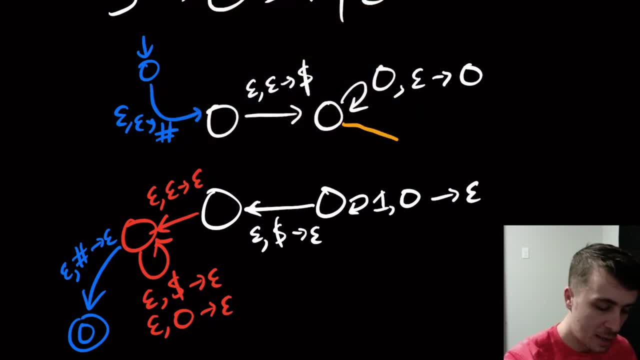 up into two different transitions. So let's say I have a new state right here and the trick was to push something on and then pop something that the same thing off. So let's say that we're going to push a zero on. There's no reason to add another symbol to the stack. but you could if you wanted to. 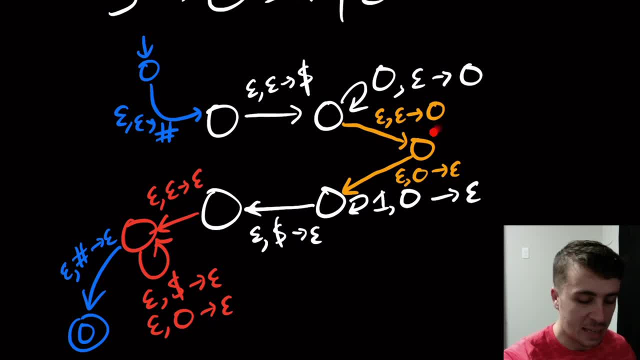 But then if you did add a new symbol here to the stack, like X or something, you would have to add another transition here. but that's totally okay And we'll do the same thing for this transition right here. So let's erase it, add a new state here and then let's do the exact same thing as. 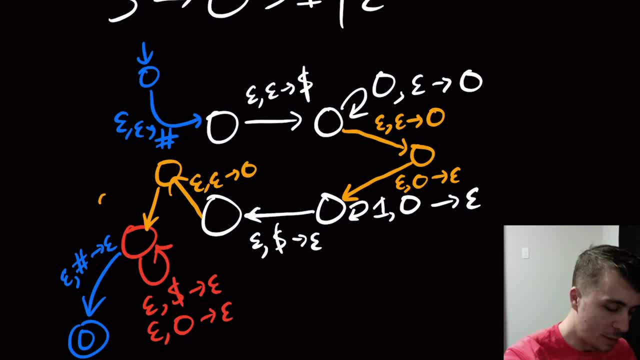 before. It doesn't actually matter which way you do this, Sorry, it doesn't matter which thing that you put on the stack here. that's what I meant to say. Okay, so I claim that this is all that we need to do, All that we need to do. But yeah, so every state, sorry, every transition pushes, or? 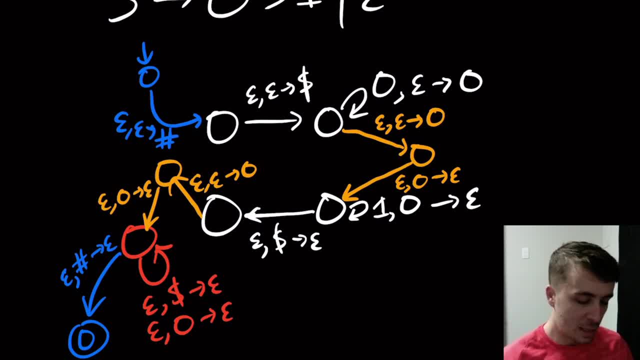 pops something, It doesn't do both, And there's a single final state down here and we ensure that the stack actually does end empty. So let's give these states names: q0, q1,, q2,, q3,, q4, q5, q6,, q7,, q8.. 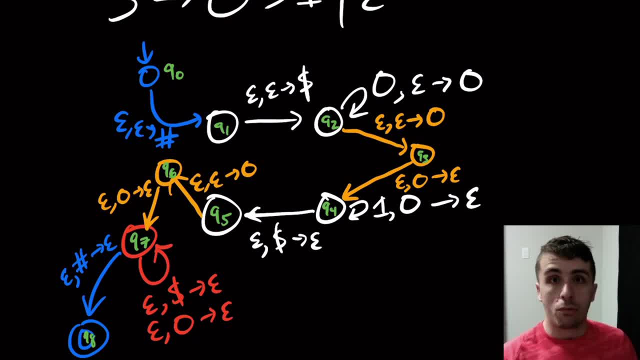 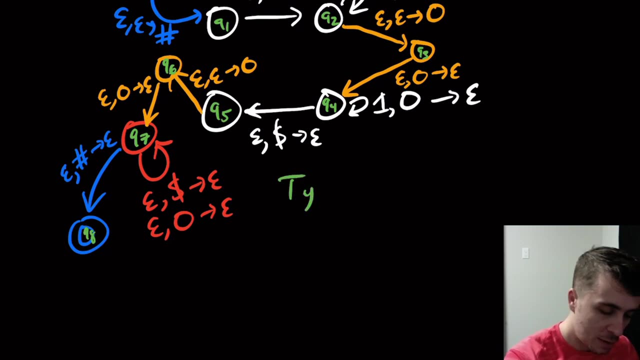 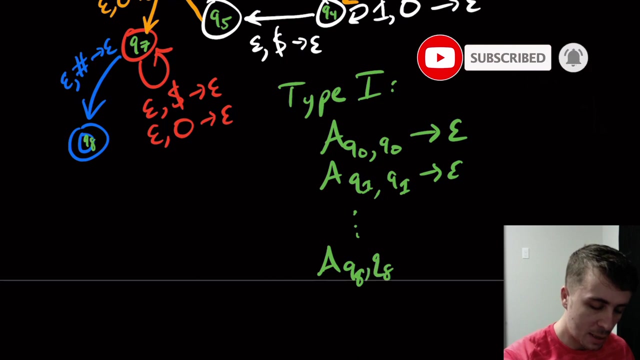 So we, if you recall from what we did before, the first type of rule was to have a sub any state comma, the same state, going to epsilon. So for type 1 rules we will have something like a q0, q0 goes to empty, a q1, q1 going to empty, etc. up to a. make sure it appears q8, q8 comma goes to epsilon. So we'll have 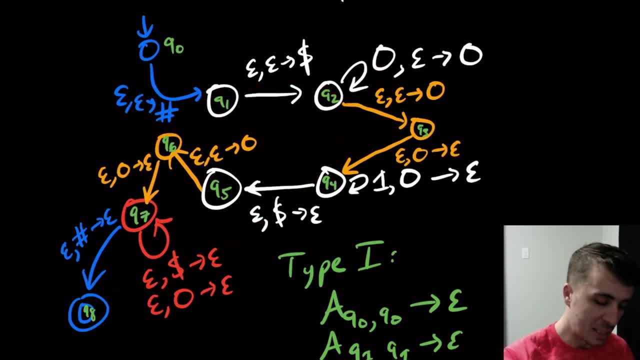 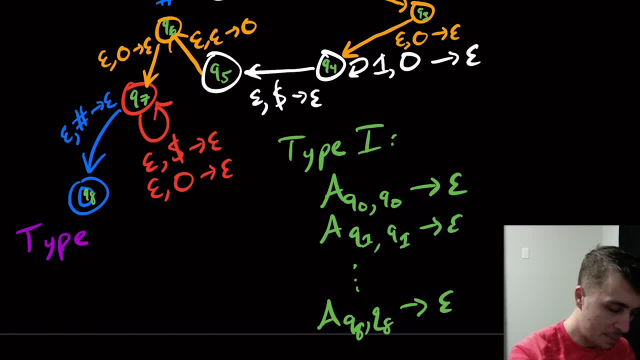 nine rules right here, because there are nine states, And then for type 2 rules- type 2, we will have something like a some state, some state going to two variables over here, where the one on the left, so the variable on the left, it has two subscripts, The one on 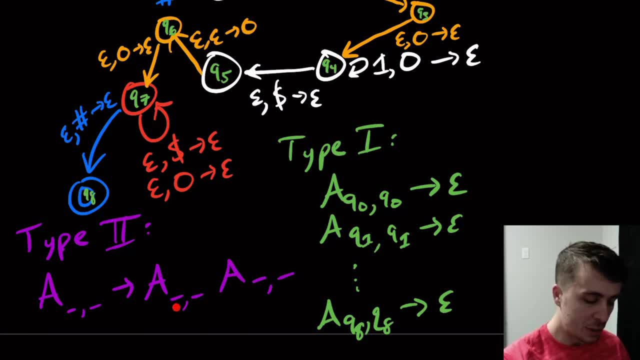 on the left is going to be the one that appears in the first variable on the left. the second one over here is what appears in the second variable on the right, and the two in the middle have to be exactly the same because we wanted to go from one state to some intermediate state and from that. 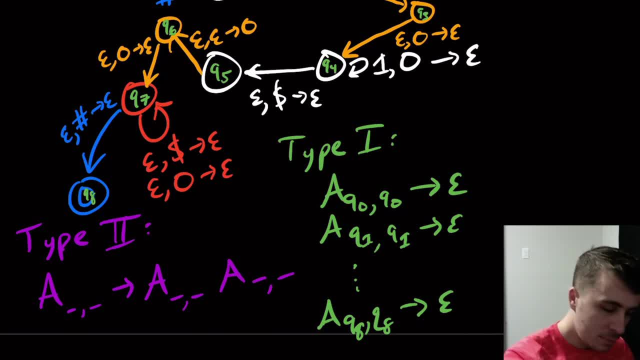 intermediate state to the end. So, as an example, what we could do is that we could do, let's say, q0, q7, so that means I got to put a q0 here and a q7 at the very end, put some commas in and I can. 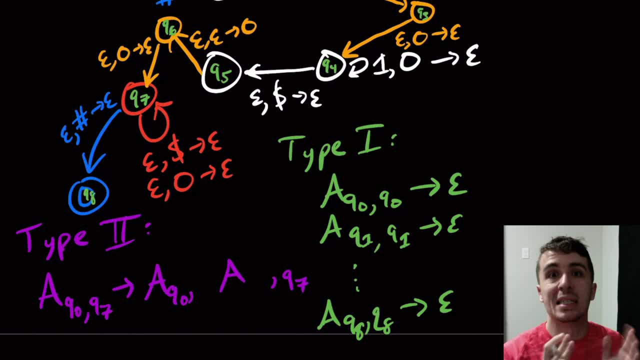 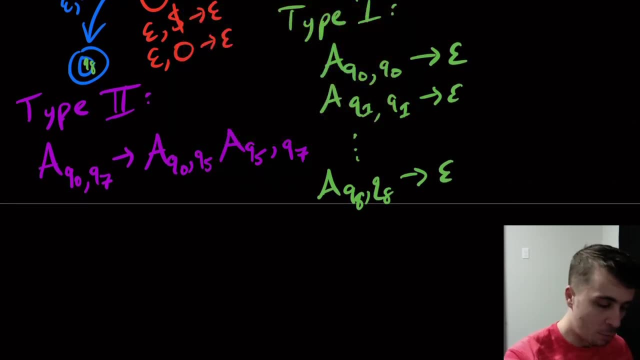 put any state in the middle that I want to, as long as this is the same for both. So let's say I put q5. That's totally reasonable. And it could be that one of these variables makes no sense. So, for example, this one won't make any sense. So let's say q0, q3 goes to a q0. That's, it still has to. 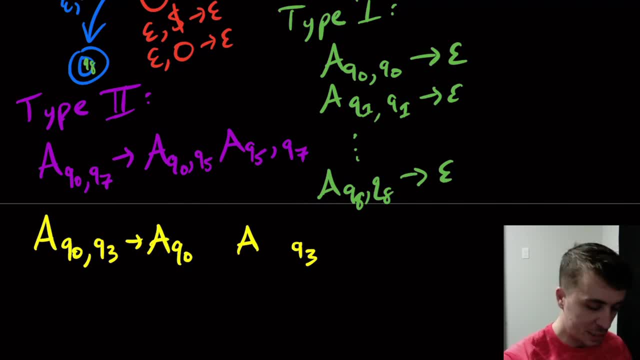 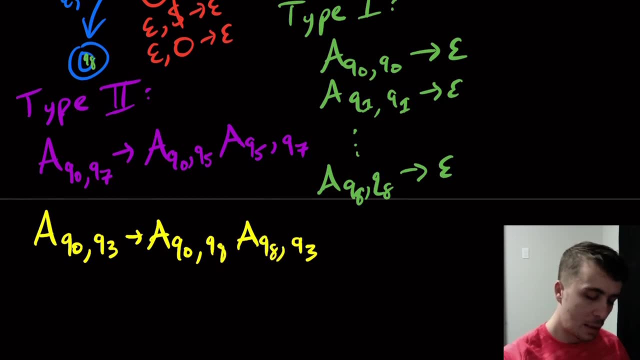 appear there. q3 has to appear at the end because that's what the left variable tells me. And let's say I put q8 as the intermediate state. That's a total reasonable state. So I can say q8 is a totally valid rule and it's one that I will put in, but it makes no sense for. 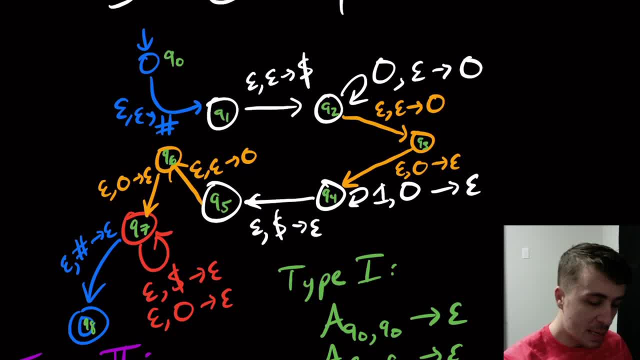 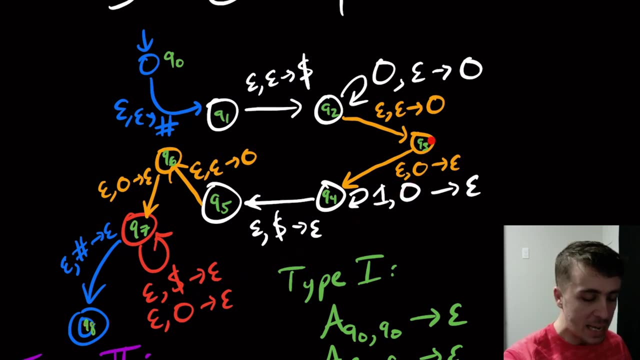 this particular PDA? Why? Because it's asking what strings take me from q0 to q3 right here. But it's saying one route to go is to go all the way down to q8 and then from 8 to 3. But there's no path. 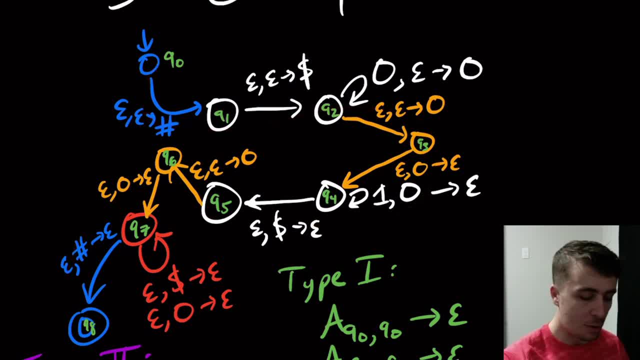 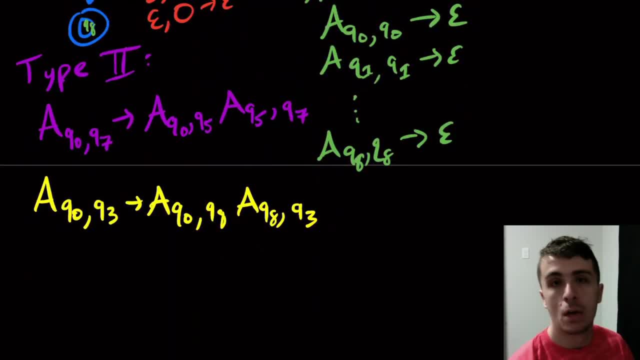 from 8 to 3.. There is from 0 to 8 going through the whole thing, but there's nothing from 8 to 3.. So, in fact, this variable right here will not actually generate anything, And that's okay If I. 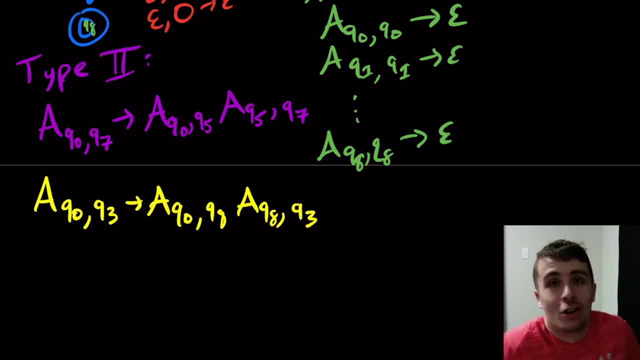 put a useless rule in. it's not going to help, It's not going to hurt, It's not going to help either. But by putting this in I don't have to think anything about the PDA itself. I could be entirely algorithmic here. Okay, so this is a rule that we'll add in. and this is a rule that we'll add in. 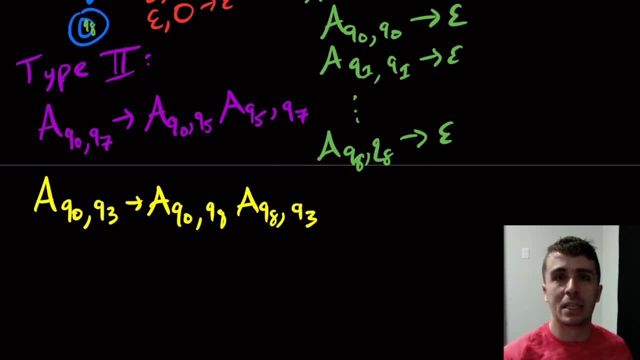 We'll add in all 727 other rules. So this is a rule that we'll add in. We'll add in all 727 other rules. So this is a rule that we'll add in and this is a rule that we'll add in. We'll add in all 727 other. 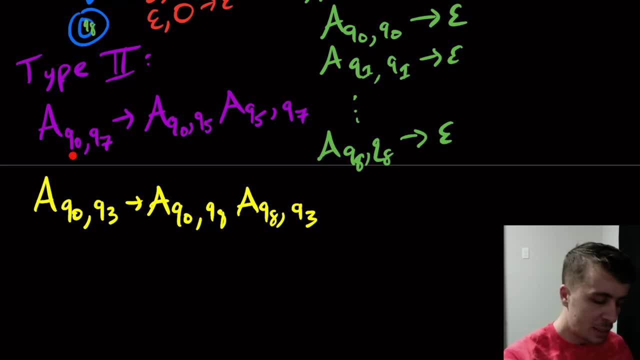 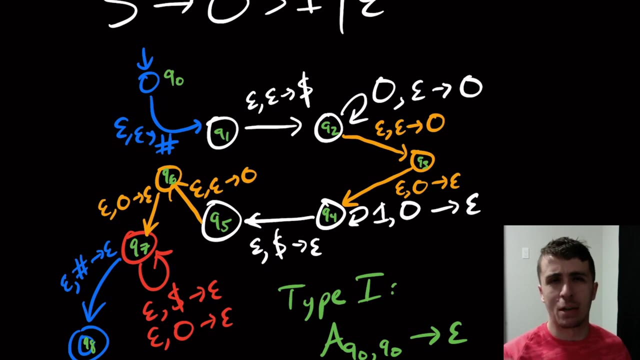 rules. How do I know that's the number? Because for each of these subscripts right here- So this one, this one, and then this is the third one- I have nine choices for each one of them, Because there are nine states in the whole thing And they could be the same, So it's not like one has to be. 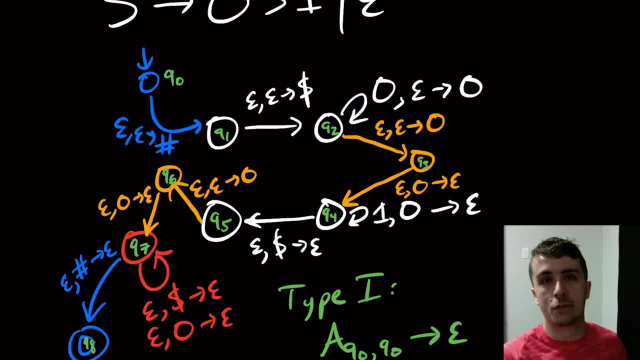 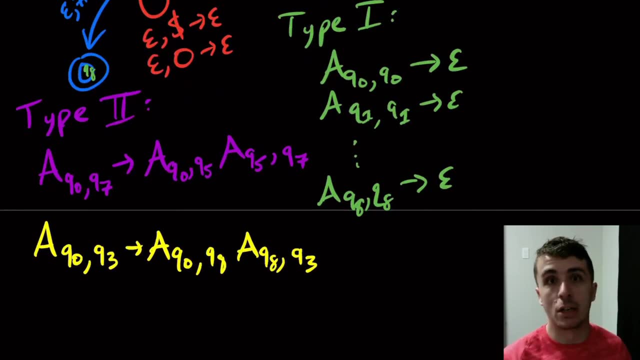 different. So I have nine times nine times nine different rules. Actually, no, it was 727, not 725.. So there are 729 total rules. So there are 729 total rules. So there are 729 total rules. So here we have 9 more rules that are going to be made this way, and I made two of them, So there. 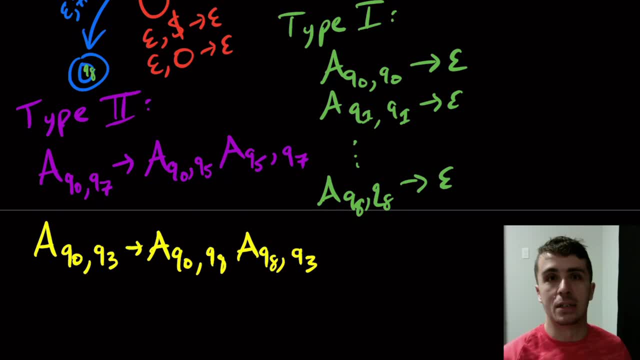 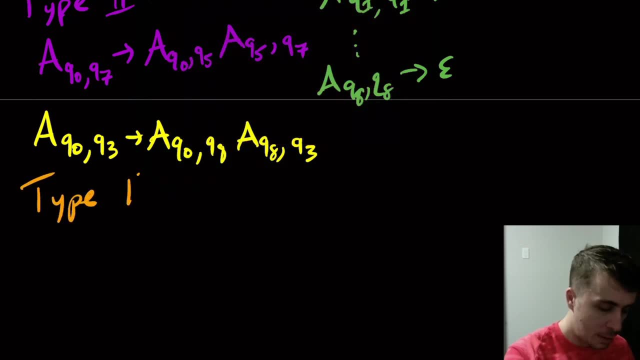 will be 727 more. But it's easy to make all these rules. You could just make three, four loops and then you're done, Alright. so let's look at a Type 3 example. So remember, for Type 3 you need to have a pair of matching transition ones, that one pushes something and the other one 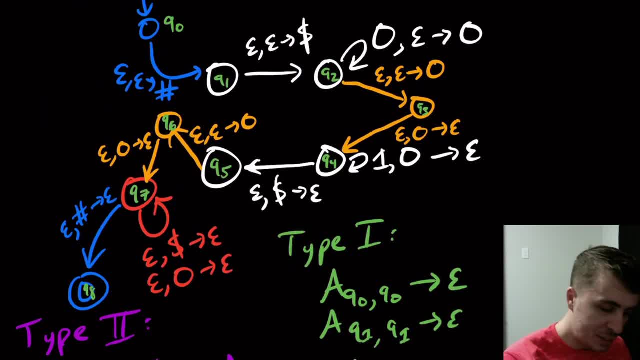 that there exists a pair, because this little step right here which allowed us to pop everything off. so as long as the PDA actually pushes something at some point, then we will have the match right here, but if it doesn't, then the PDA is actually really simple, because if it has no pushing transitions, it can't execute. 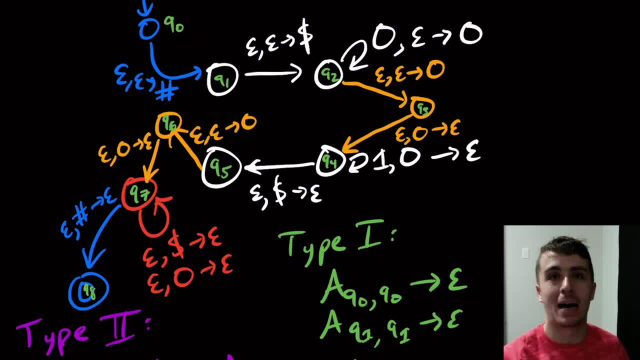 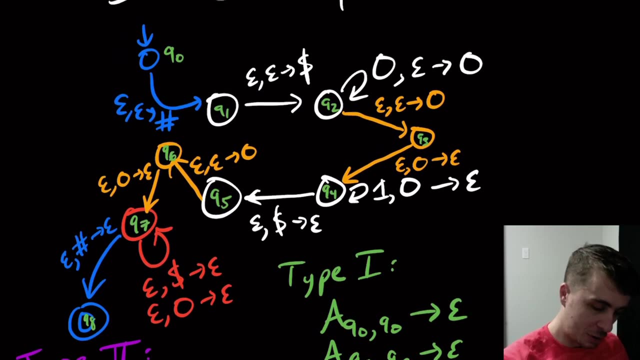 a transition, because every transition either pushes or pops. and if no transition pushes, every transition then pops, which means I can never leave the start state or execute any transitions. okay, so let's look at a matching pair of transitions. so let's say we will look at the beginning and the end transition. so 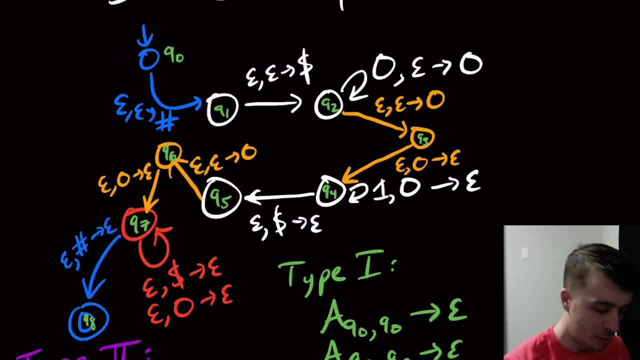 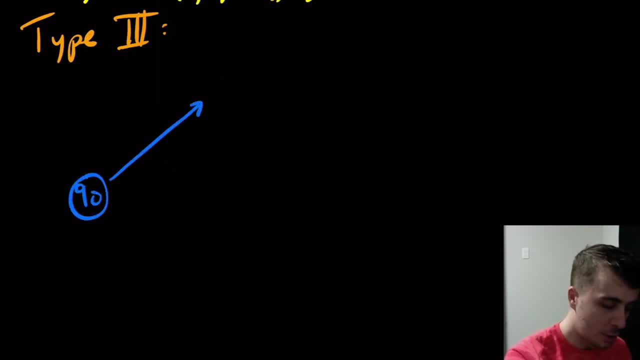 this the, this blue transition, and then this one, and I'll put them down here so it's easier to see. so we have Q0 here going to Q0 here going to Q1, and that transition is pushing on the dollars, the pound sign and the last. 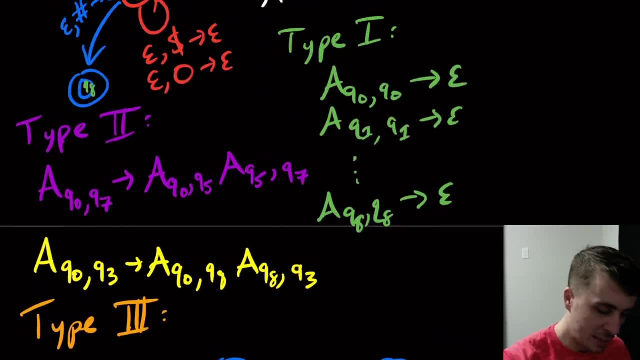 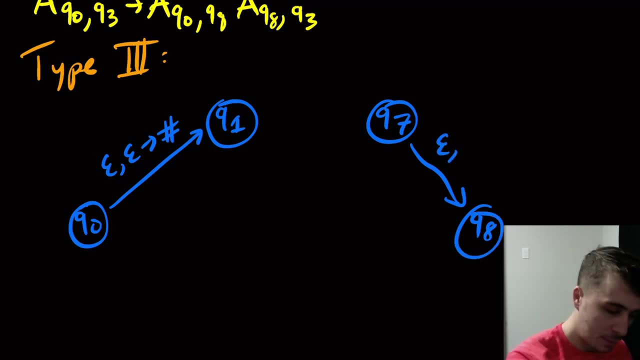 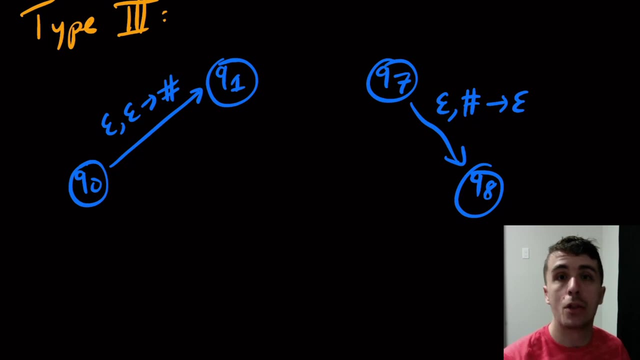 transition. is Q7 going to? I think it's Q7. yeah, it's Q7 going to Q8 over here and we will be popping off the pound sign and I could have equally chosen the other any other transition that happens to have a pound sign, but these. 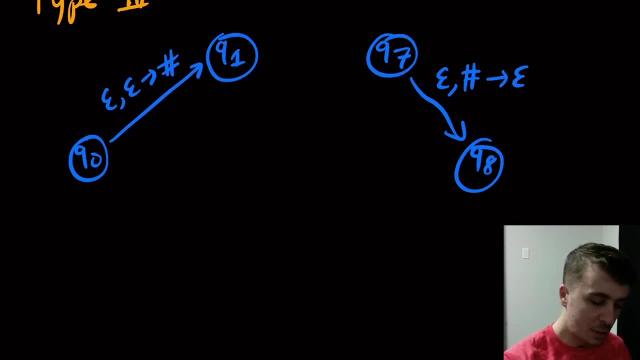 are the only two that happen to have it at all. all right, so what's the recipe here is? I want to get from Q0 to Q8, so from the pushing one, I start from the start, the state that is the beginning of the transition, which is Q0. and I want to get 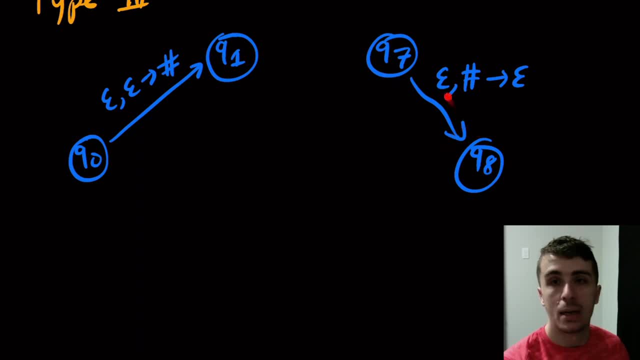 to the state. that's the end of the popping transition. so the rule we'll be adding is AQ0 to Q8. that's my start and my goal. then what do we read on this transition? well, it says nothing, so I don't put anything right here. then whatever takes me from Q1 to Q7, so AQ1. 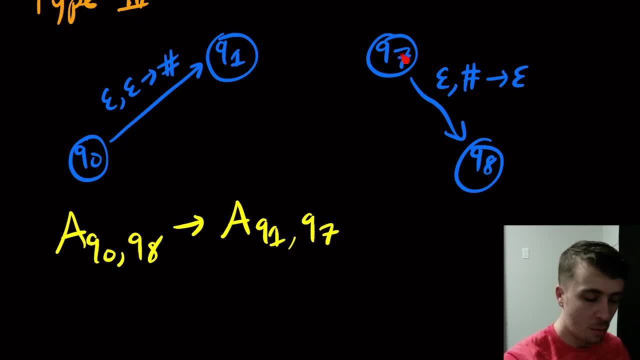 Q7, and then how do I get from 7 to 8? well, I don't read anything there and so I don't put anything here. so this is the entire rule that is actually made here. so look, okay, so let's actually do this. so let's actually do this. so let's actually 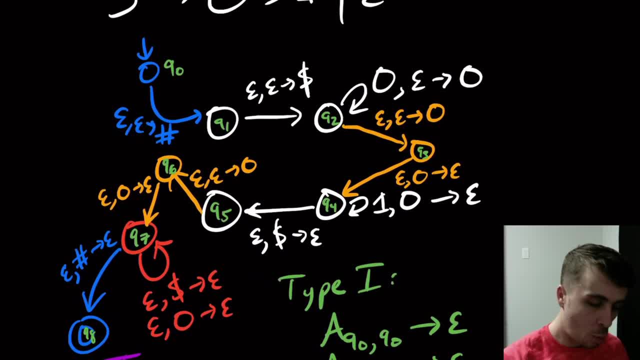 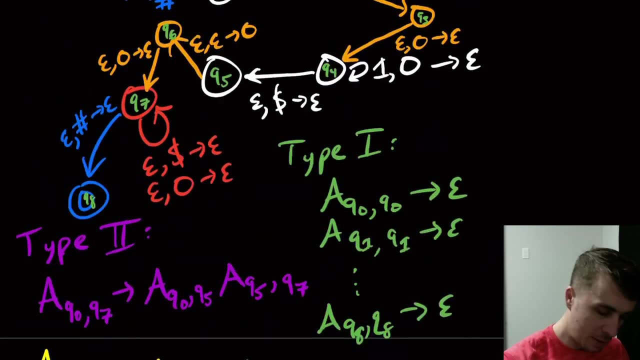 do a different example. let's do one where one reads and the other one doesn't. so this one pushes a zero on and this one put pops off a zero. so let's look at that example. so I think that state was Q2, so I'm gonna draw it a. 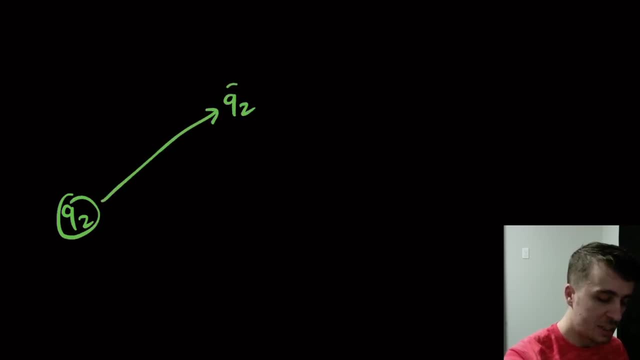 little differently, I'm gonna have at the same. it looks the same, but note that these two states are the same. because they're the same states and they're the same because it's a self loop in the PD gate, I'm gonna draw it like it isn't a. 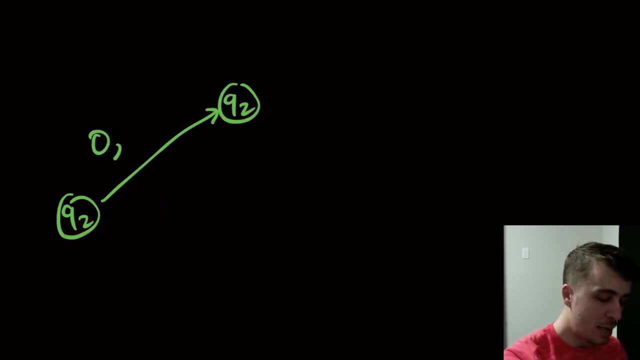 self loop so it's easier to see. so this one read a zero, pop nothing, and pushed a zero. and then the other one was Q7, which was a self loop, and it popped a zero. so Q7 going to itself. so again, not drawing like a self loop here, and we will not. 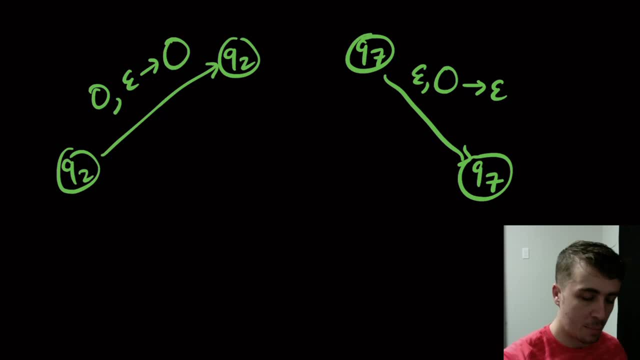 read anything, pop the zero and push nothing. so the recipe, of course, is going from the beginning of the push guy to the end of the pop one. so that's a Q2 to Q7. what did we read on the push transition? we read a zero. whatever takes me from two to seven. so it's the same variable here. 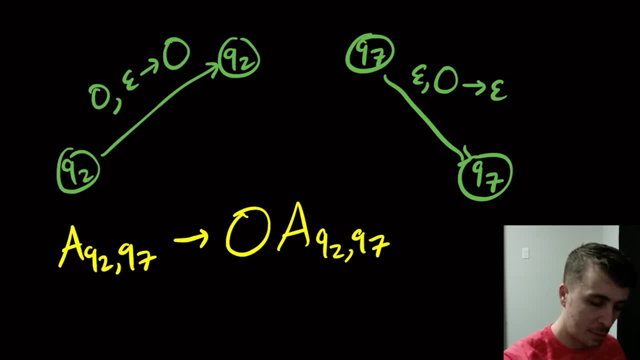 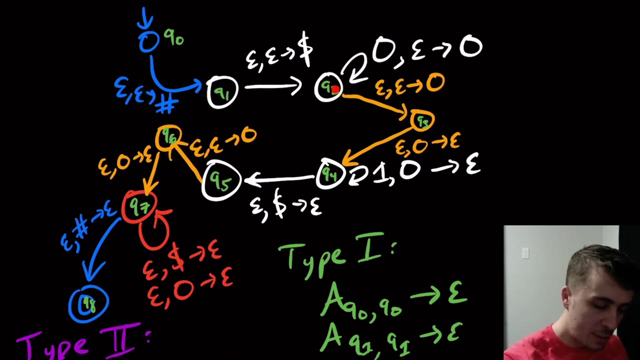 a Q2 to Q7 and nothing read on this one, the pop one. so I don't put anything here, and so this is the rule that will actually be made and you can actually kind of see why this works, because whatever takes me from here to here, I 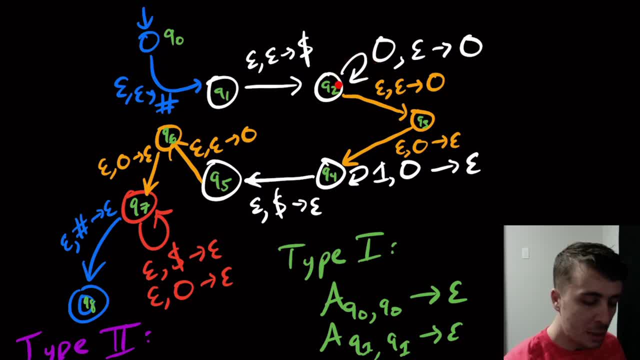 could read a zero and then just ask the question: how do I get from two to seven? okay, and because the push was done here and the pop here, we can ask the same question again. so this zero? because there's a self loop here that says that or implies that this rule works, because I can just read a zero and then ask the? 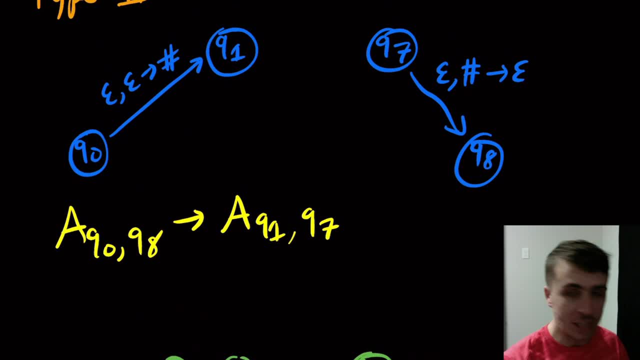 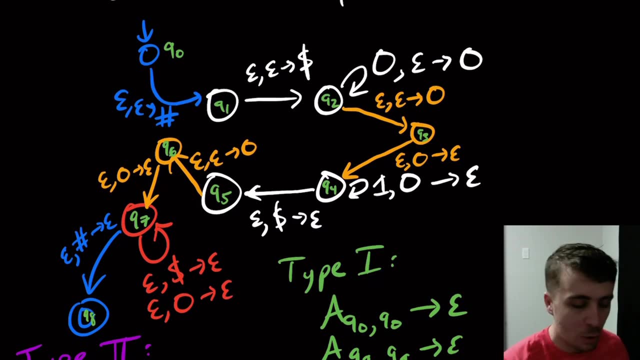 same question, again from the same variable, because we're effectively just starting from wherever we just left off. all right, let's do one, the only the only one, where we read on both transitions. so this one reads a zero, this one reads a one and they are matching, because the thing that's pushed 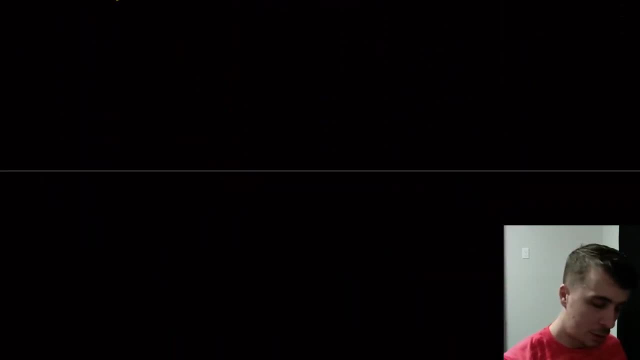 here is the thing that's popped here. so let's, let's actually look at that. so I know the first one's Q2, the second one is Q4. all right, so again we have Q2 going to itself, which is zero, epsilon goes to zero, and then we have Q4 here going to Q4 on reading a one, and then 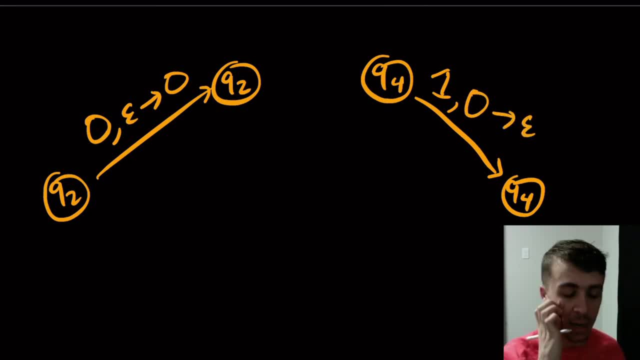 popping the zero off and pushing and pushing nothing. so if we follow the recipe, we want to get from two to four. so a Q2 go going to Q4 going to Cali. so what did we read on this one? we read at zero and then whatever we took, 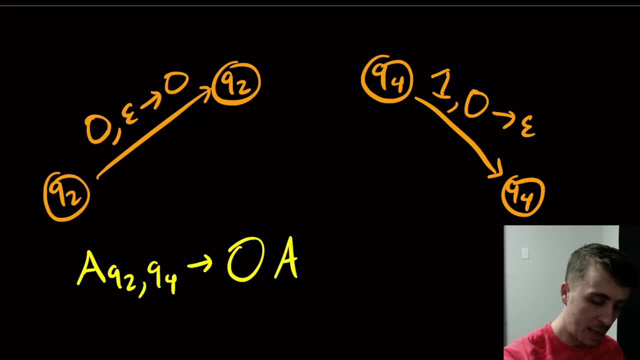 whatever takes us from two to four, so a Q2, Q4. and then what if we read on this transition, which is a one, so you can actually kind of see the internal, the internal grammar that we usually use to create the four, one, four, zero to the end, one to the end, because this is almost identical to s going to zero s one. 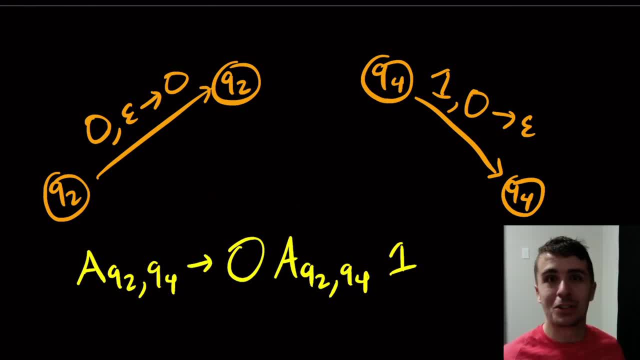 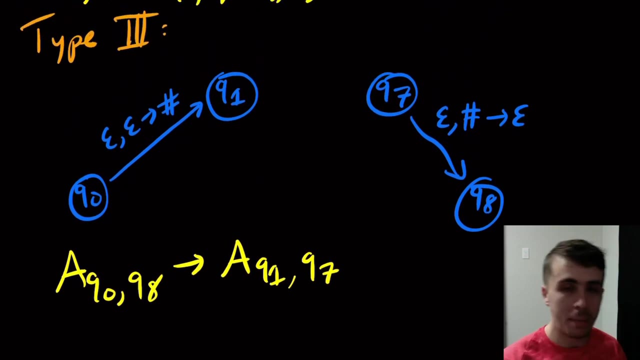 it's just that a lot of these other variables are going to either generate nothing or the empty string, so so you can kind of see this actually occurring here, or there's a bunch of unit rules too, and in fact we saw that right here. there's going to be a lot of unit rules because pretty much every